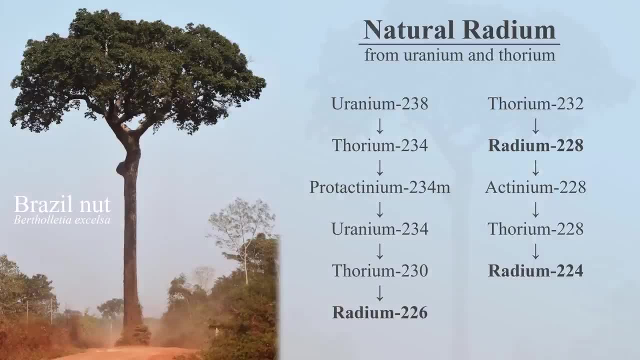 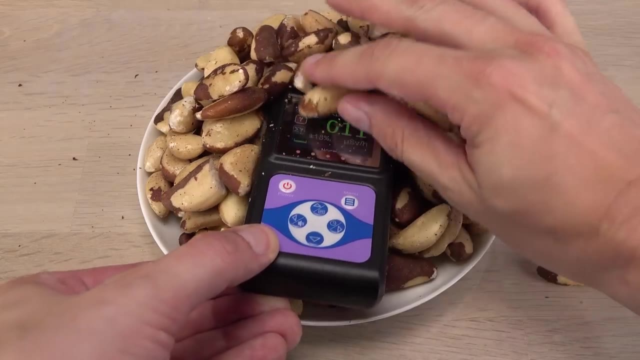 And Brazil nuts come from one of the tallest trees in the rainforest, A tree with an extensive root system reaching a lot of soil, with natural radium from uranium and thorium decay in the ground. However, I'm still not detecting anything. Why would bananas and Brazil nuts even be considered radioactive then? 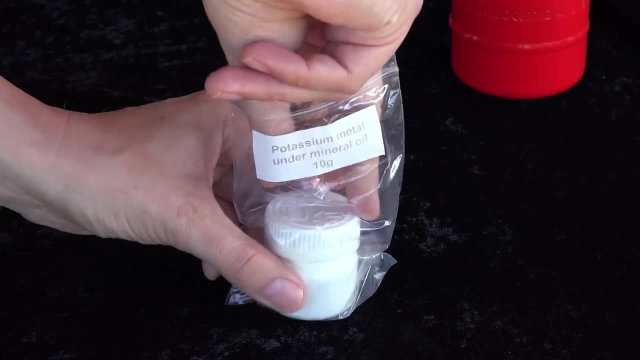 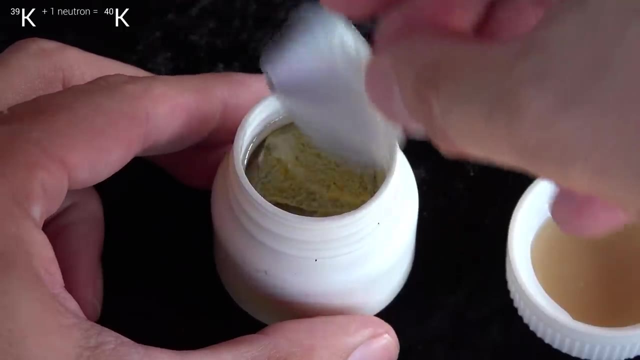 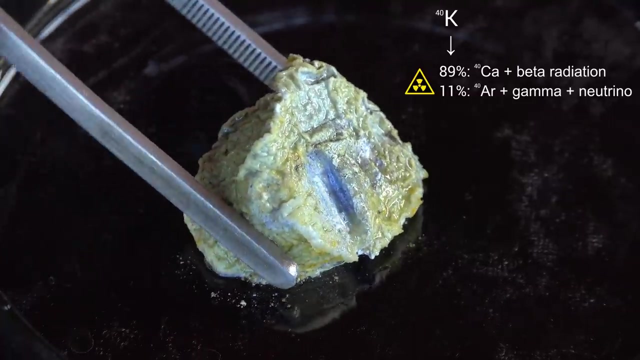 The main reason is a metal called potassium. Potassium is essential to life, but a tiny part of natural potassium is special because it has an extra neutron in the nucleus: Instead of 39 nucleons, it has 40.. It is known as potassium-40, and this is unstable. 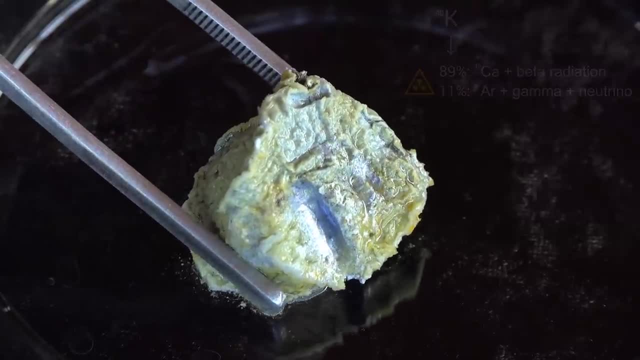 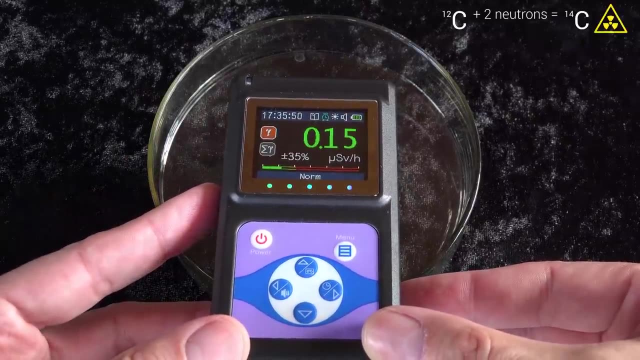 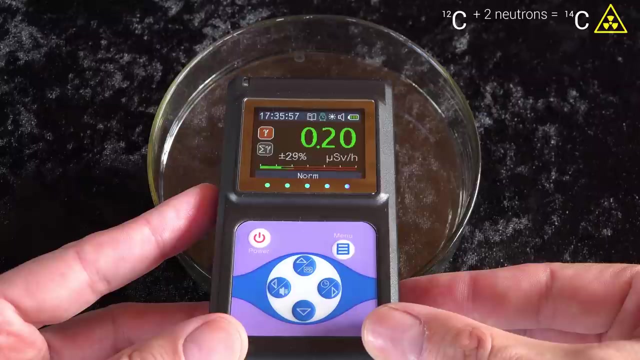 Radioactive, So anything containing natural potassium will be slightly radioactive, including bananas, Brazil nuts and your body. They also contain carbon. An element which also has a lot of potassium Also has a natural radioisotope with an extra neutron in it. This is known as carbon-14. 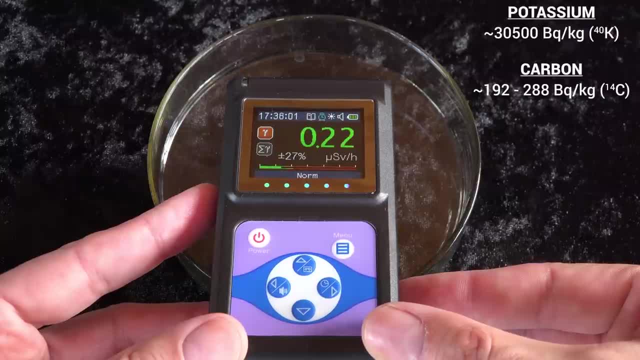 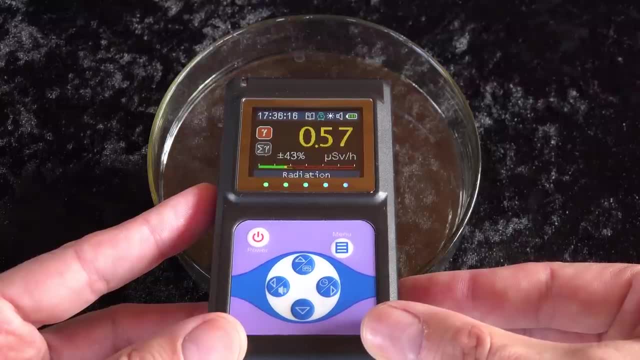 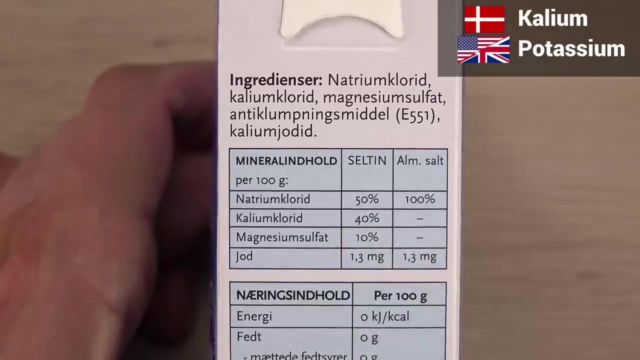 But potassium is by far the most active, so I'll focus on that. Here I have some low-sodium salt, where 40% of the usual table salt sodium chloride has been replaced by potassium chloride. It even contains a tiny amount of potassium. 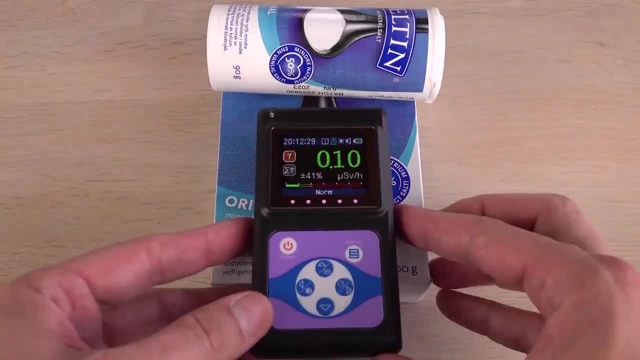 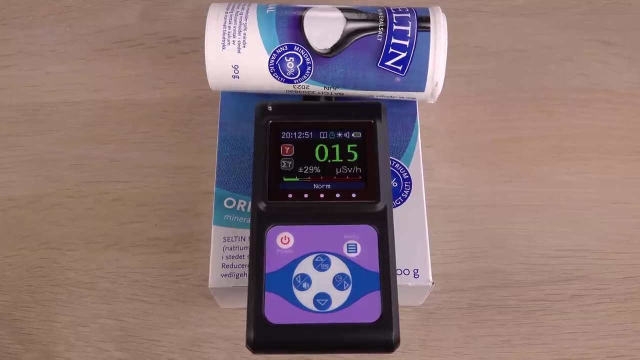 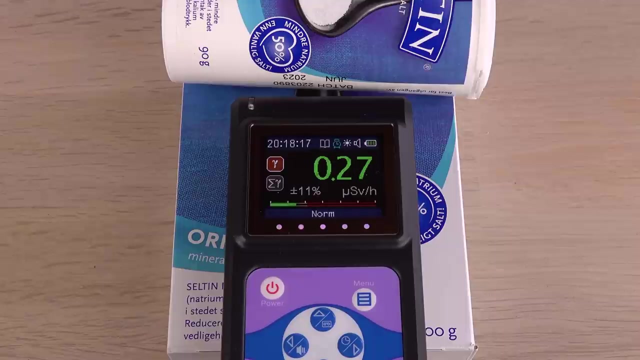 This low-sodium salt is way more rich in potassium than the foods I have shown so far. Let's see if the Geiger counter can detect it It does. 0.27 micro sieverts per hour in average is more than twice as much as my usual background radiation. 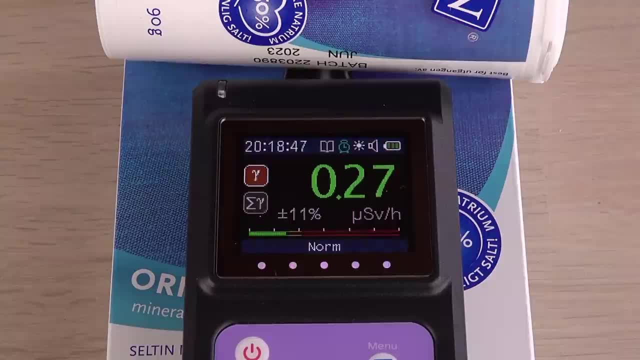 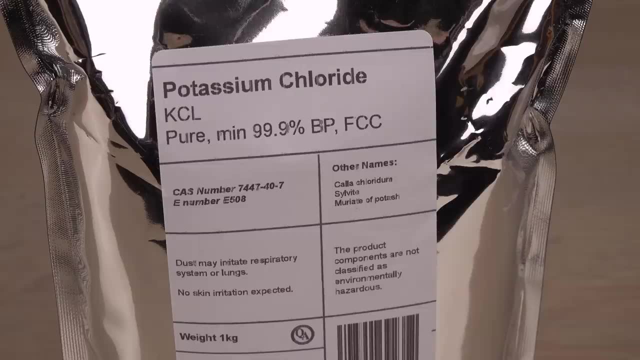 At the higher concentration the potassium is detectable, with a Geiger counter Going even higher in concentration. you can buy salt substitute where all of the sodium is replaced by potassium. I couldn't find an example in the local stores, but this bag contains 1 kg of 99.9% pure potassium chloride. 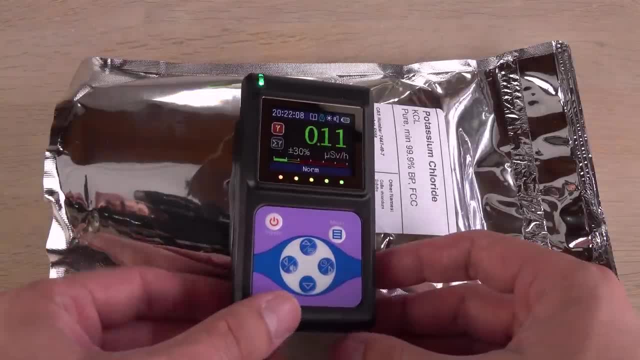 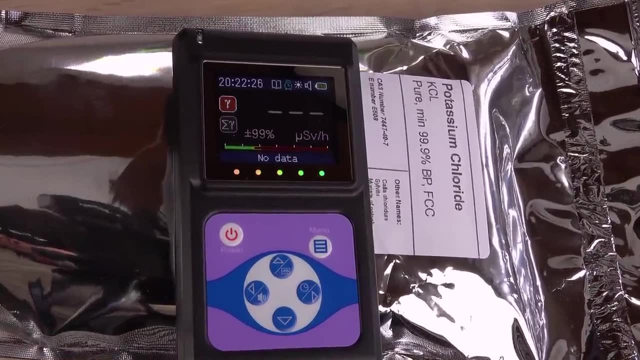 known as food additive E-508.. Surely the Geiger counter will detect the potassium in this. Aww, yes, This is around 5 times the background radiation at my place. The Geiger counter sent out an SOS telling me something more radioactive than normal is near. 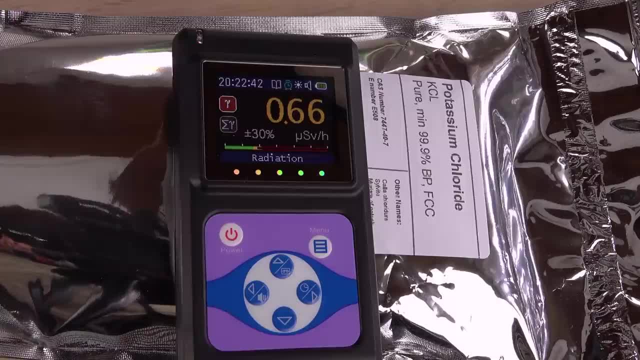 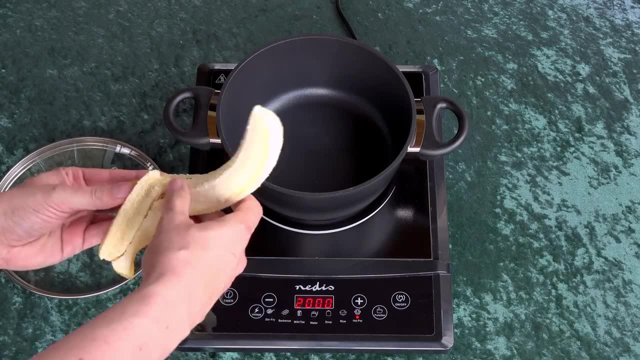 Not surprisingly, the higher concentration and larger amount of potassium, the more radioactive and easier to detect. It is therefore time to do some simple chemistry on the bananas. I need to concentrate the potassium in them. The simplest way is to remove the water content. 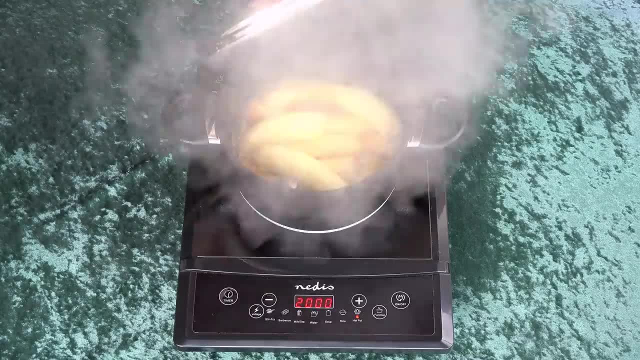 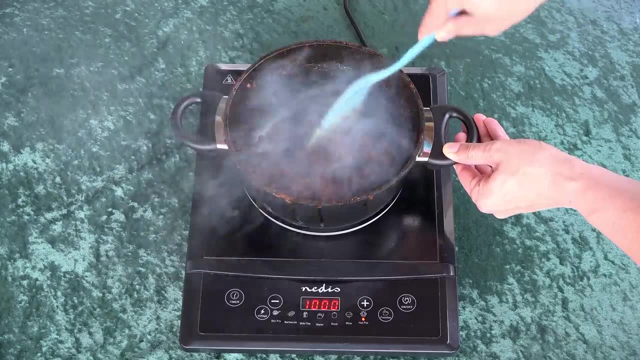 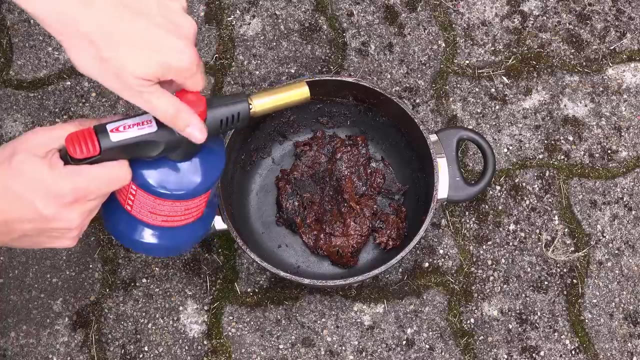 Bananas are around 75% water, so let's cook that away in a pot reserved for experiments. As the water vapor turns into smoke, the induction cooker shuts off with an error code. E-3 means the cooker is asking me: Are you sure the pot is not empty? 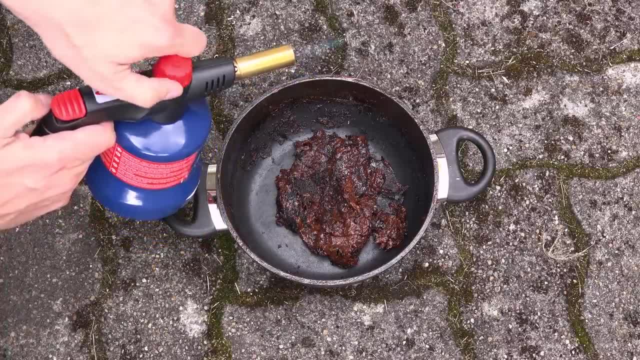 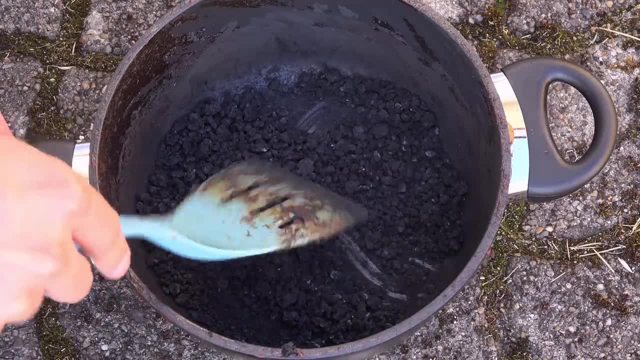 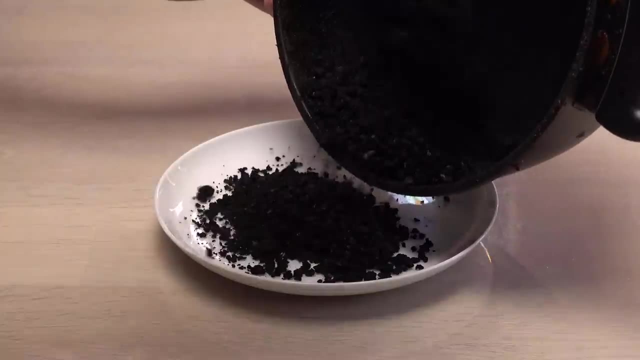 Alright, Time to go full Viking on it. No more fine Maillard reaction. Just burn it. There we have it Looking good, Not the worst meal I have cooked. Dinner is served for the Geiger counter. Will the concentrated bananas have a detectable amount of potassium? 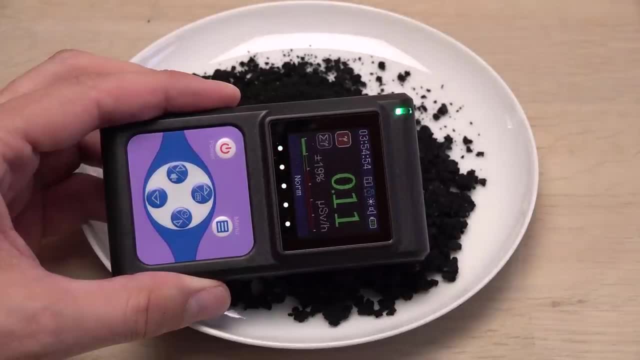 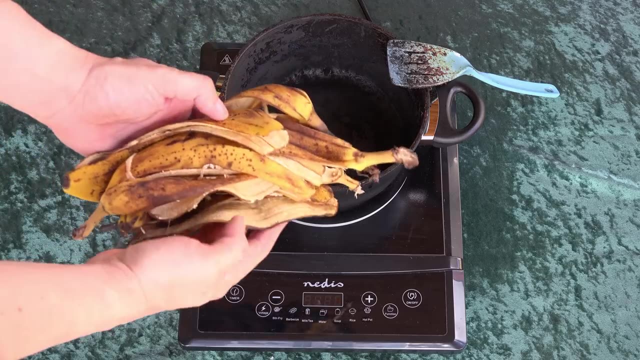 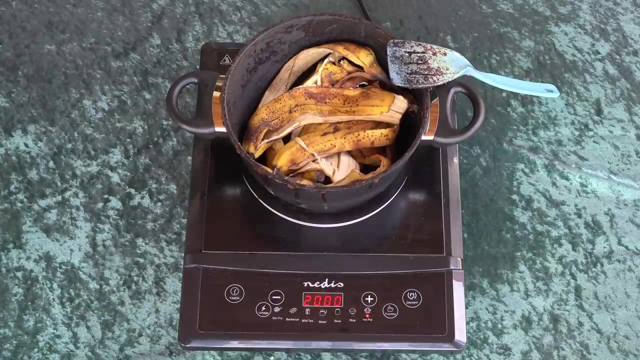 No, The radioactivity of bananas is very low, Even in concentrated form, At least on the part you eat The pulp. I got a tip that I should try testing the peel too. The peel has an interesting feature: Around the black spots there are a lot of bananas. 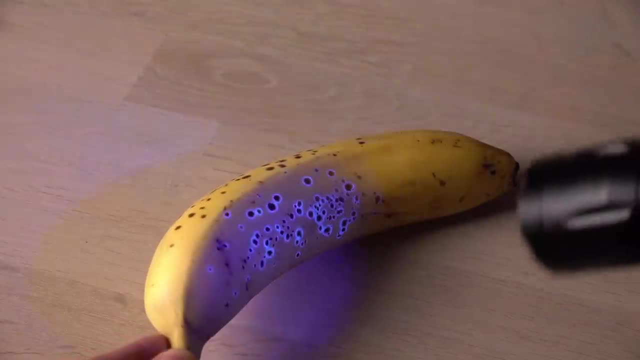 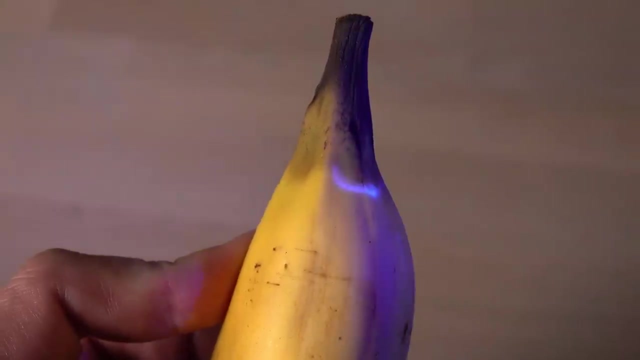 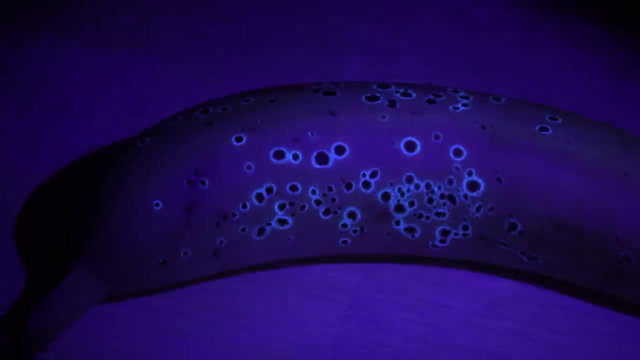 But the form. when bananas ripen, there is a fluorescent ring. Try shining a black light or an intense ultraviolet LED on it, as I do here. Anyway, this is non-ionizing radiation and not what we are looking for Before we concentrate the peels. 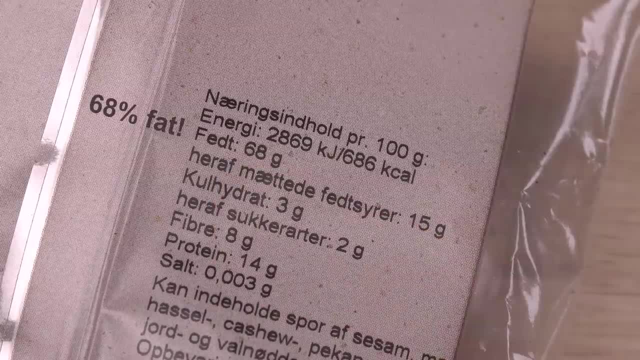 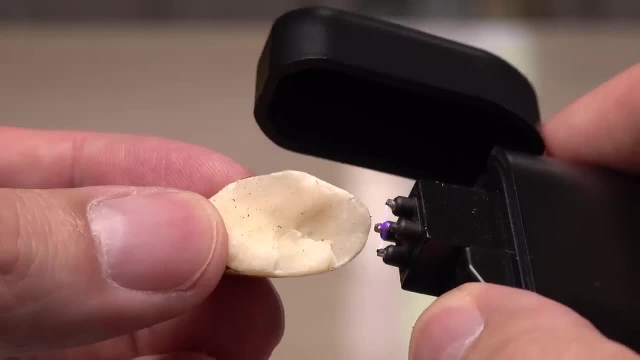 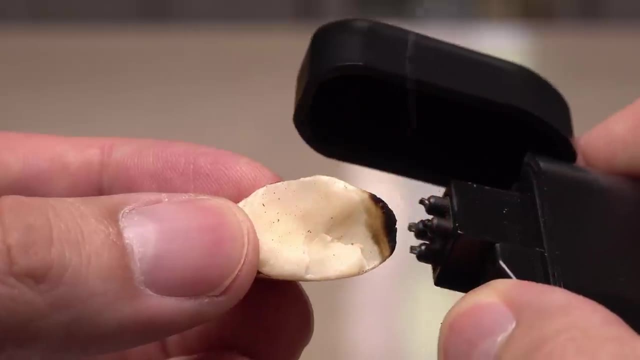 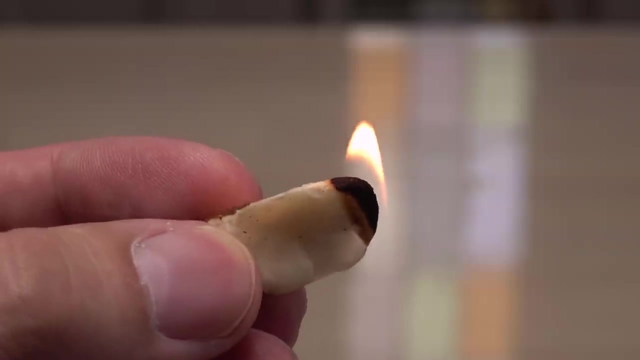 let me quickly try the Brazil nuts. Unlike the bananas, these are mostly made of fat. In fact, they are fattier than the bananas Butter I use, So you can do this. If your nuts can be lit like a candle, you may want to consider your diet. 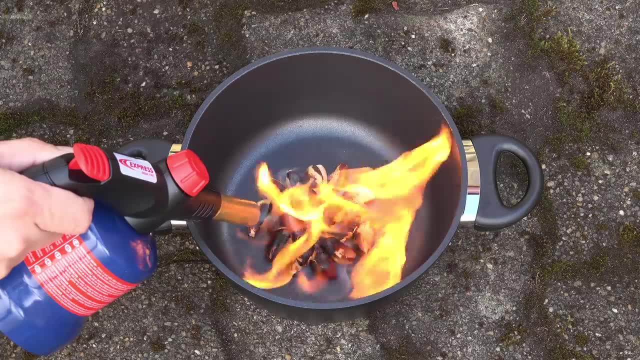 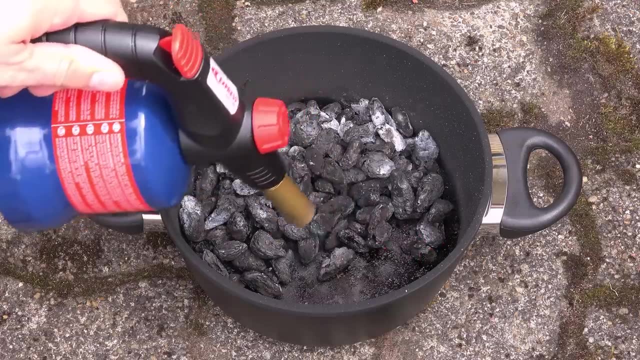 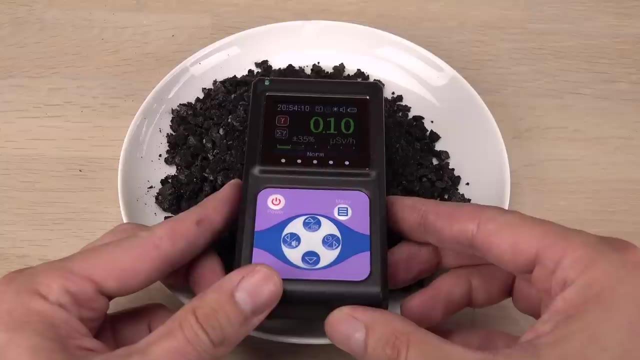 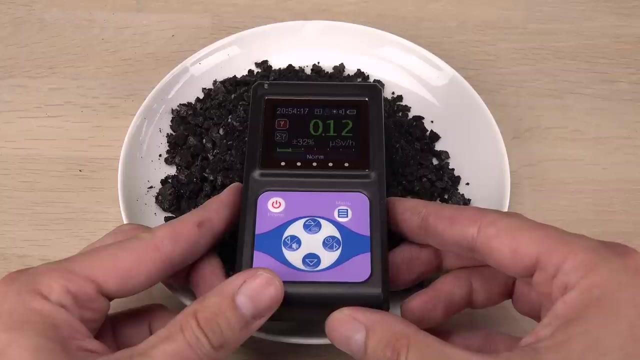 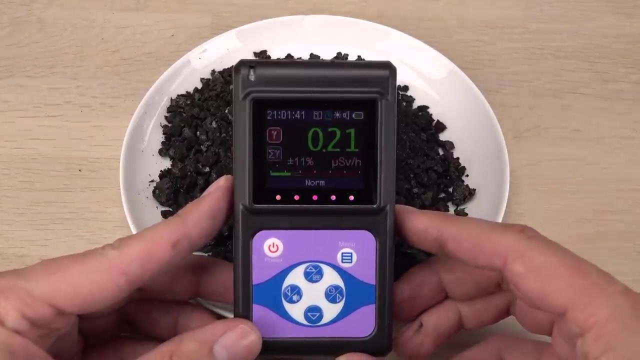 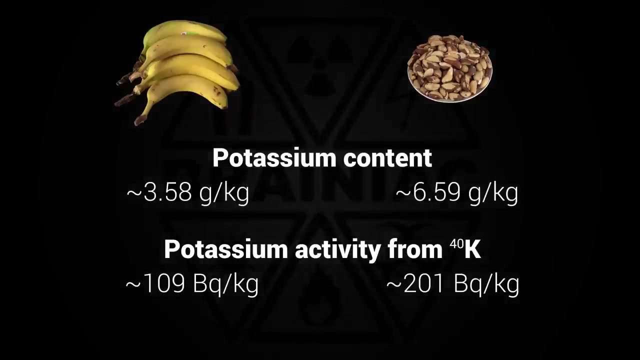 It, however, makes it easier to concentrate these. Just make a bonfire out of them After another successful cooking. it is time to test the concentrated Brazil nuts. Okay, it is a bit elevated. Most likely I am detecting the potassium, since Brazil nuts are almost twice as rich in potassium as bananas. 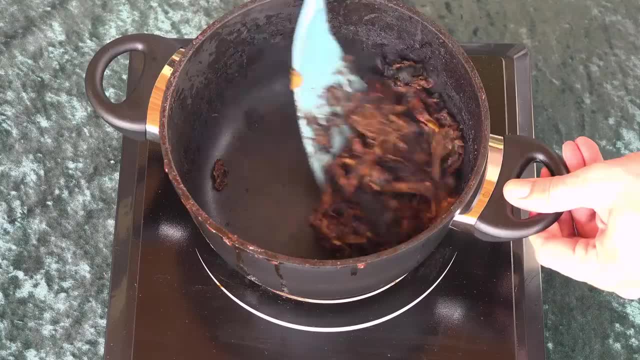 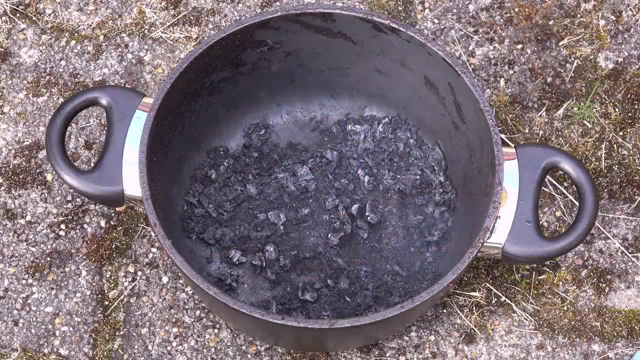 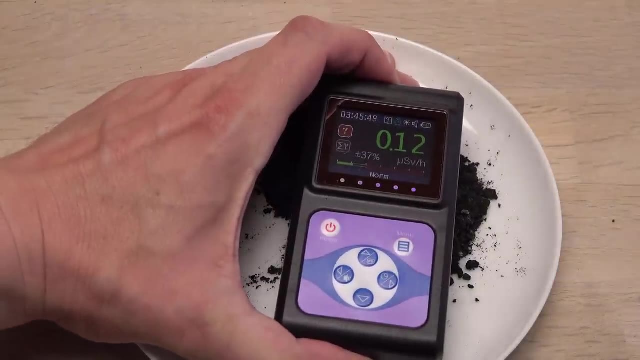 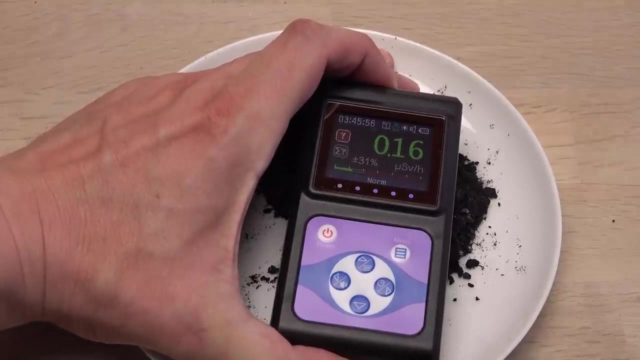 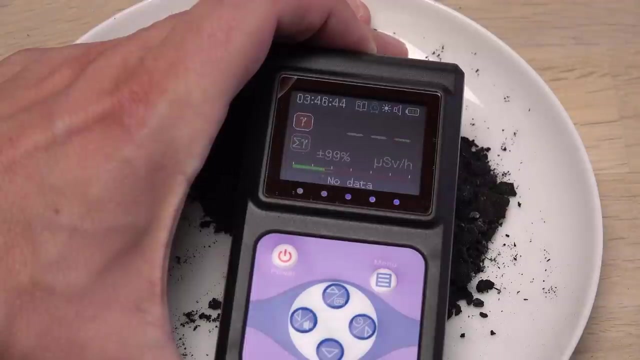 But what about the banana peels? You know the drill by now. Sounds like more clicks to me. Is it just a coincidence, A fluctuation in the background radiation, Or is it persistent? The Geiger counter has spoken. I tested it several times with similar results. 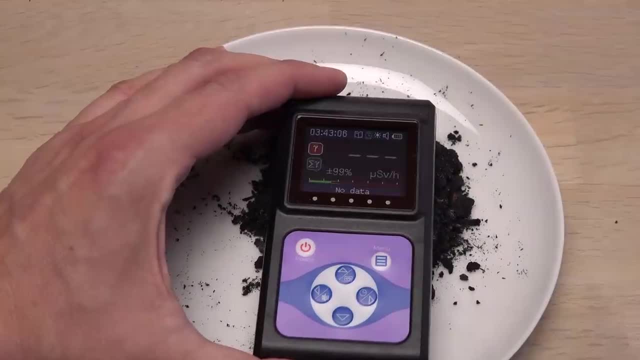 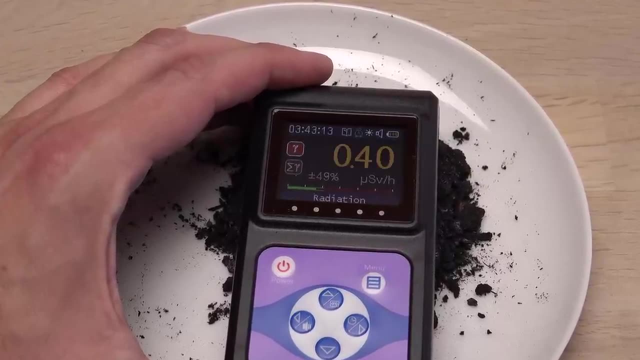 Finally, I found some detectable activity in a banana. All it took was the ash from five peels. It is known that the potassium concentration is the highest in the peels, but I am surprised to see three to four times background radiation from this small amount. 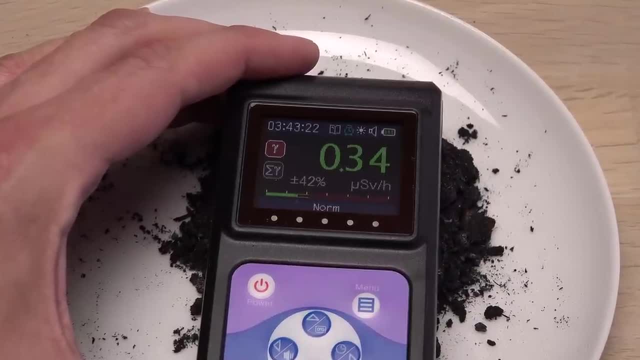 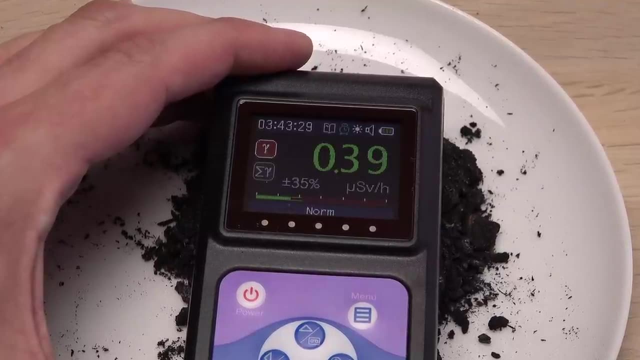 More than from half a kilogram of the low-sodium salt And more than from the ash of half a kilogram of Brazil nuts. Wish I had a gamma-ray spectrometer, I could detect what causes the radiation. You can help me save up for one through Patreon. 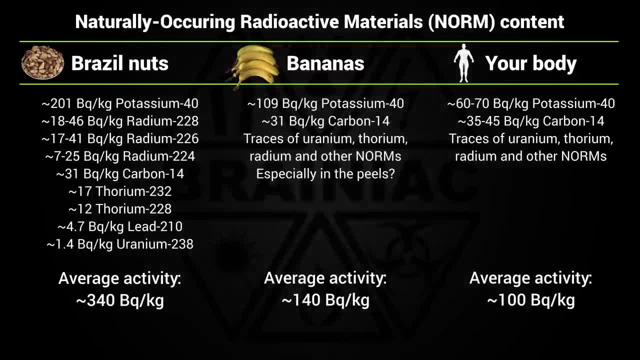 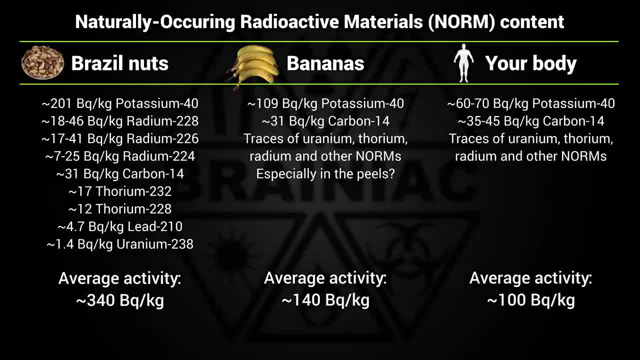 Link in the description. I do wonder if bananas gather naturally occurring radioactive materials in the peels. Anyway, I still eat bananas and Brazil nuts, and so should you. They are not much more radioactive than you are and their radioelements do not accumulate in your body. 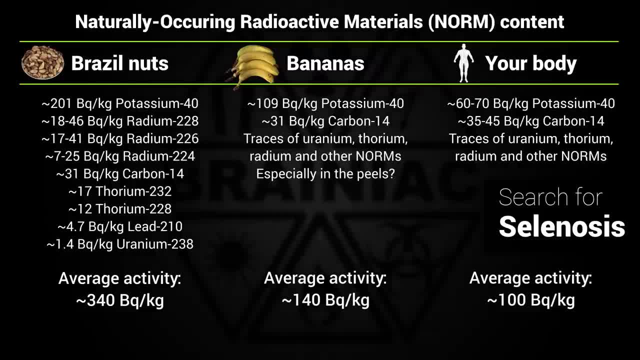 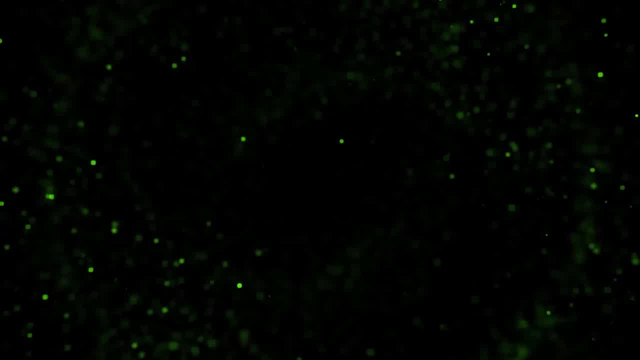 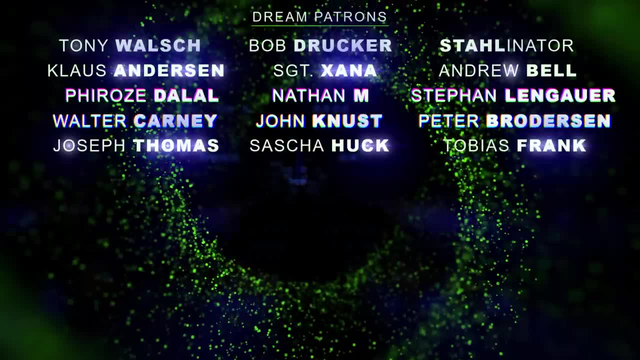 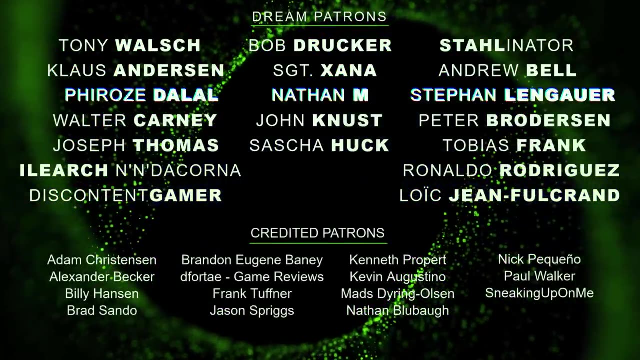 Watch out for the high selenium content in Brazil. nuts, though, Hold on for an example of something edible and radioactive you shouldn't eat. Thanks to all my patrons. I appreciate your help with saving up for the often expensive equipment. I appreciate your help with saving up for the often expensive equipment. 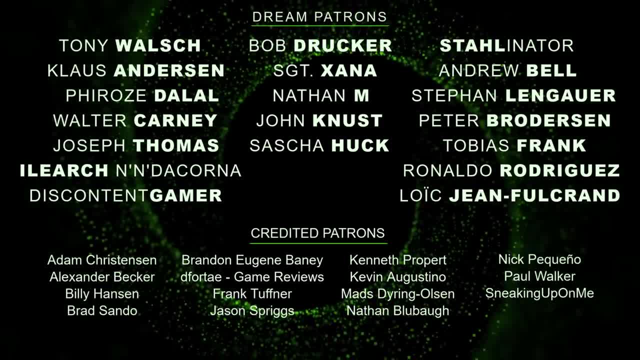 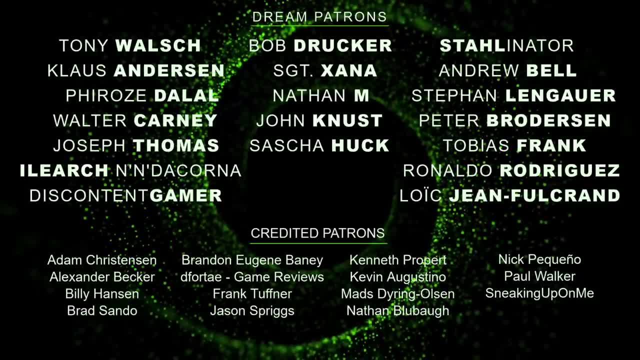 I appreciate your help with saving up for the often expensive equipment needed for my videos. Currently, a gamma-ray spectrometer is high on my wish list to figure out what is in the banana peels. You can help out on Patreon Link in the description under the video. 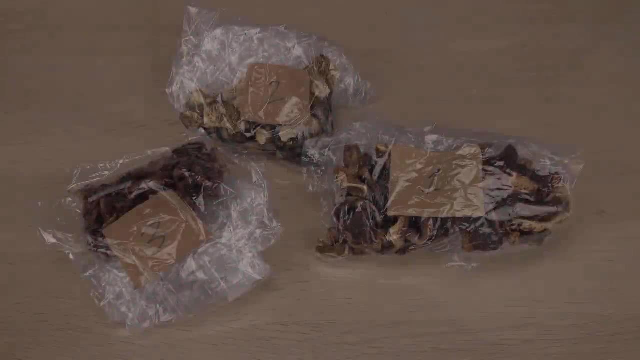 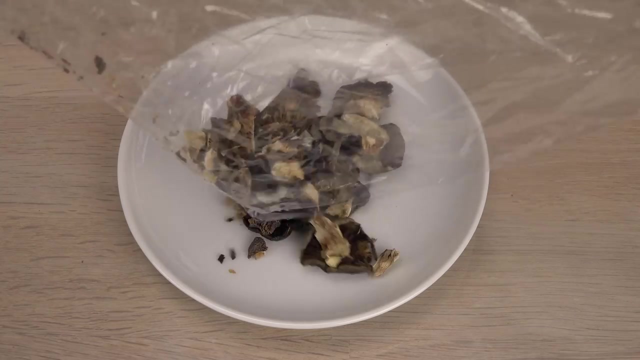 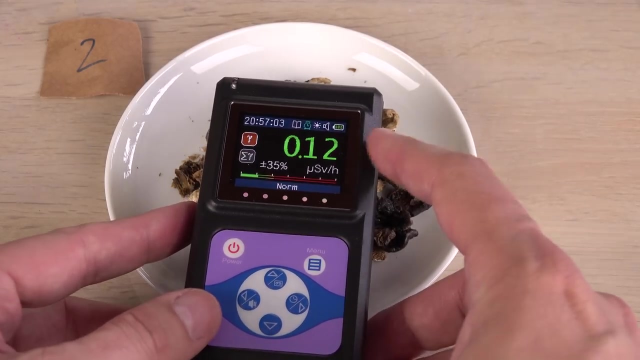 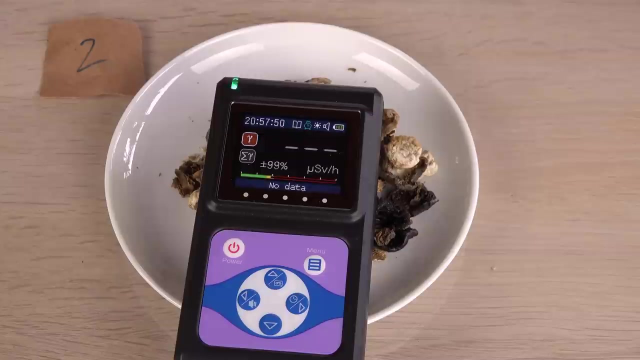 Thank you. These dried mushrooms were sent to me to try out because one of the samples is angry. They are not super hot but unlike the previous samples, there is an issue with the radioisotope in them. These have grown in the outskirts of an infamous exclusion zone and accumulated caesium-137. 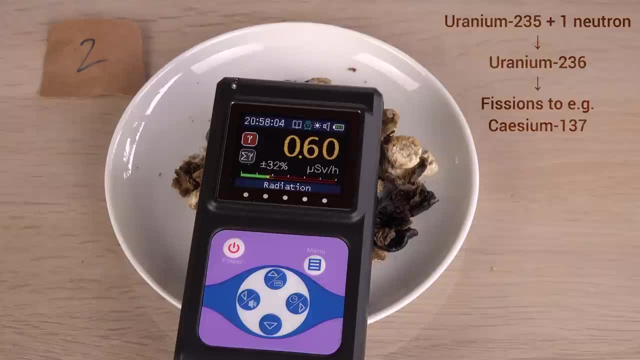 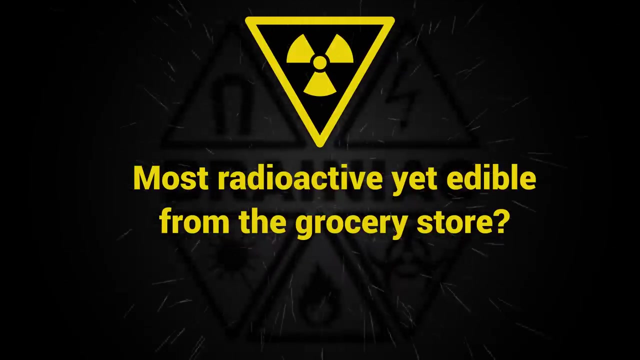 That is not naturally occurring and will accumulate in your body. So don't eat mushrooms containing nuclear fission products, please. So what is the most radioactive you can buy in a grocery store? It is salt substitute or low-sodium salt And perhaps banana peels. 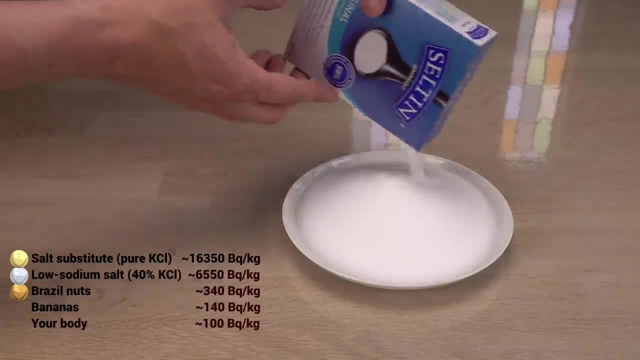 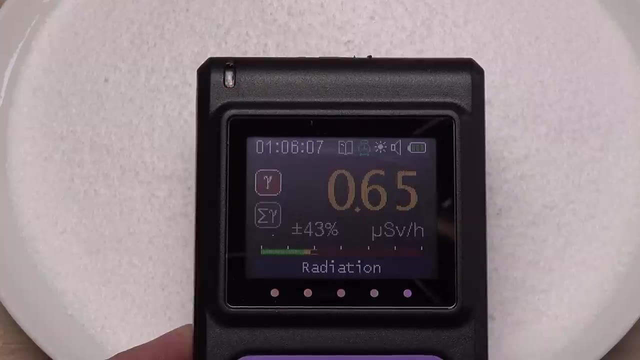 My sample of brazil nuts were not very active, but it is a natural product with great variations depending on what tree they came from. But no, brazil nuts will be stronger than potassium chloride salt substitute, making it a clear winner. I hope you enjoyed this video. 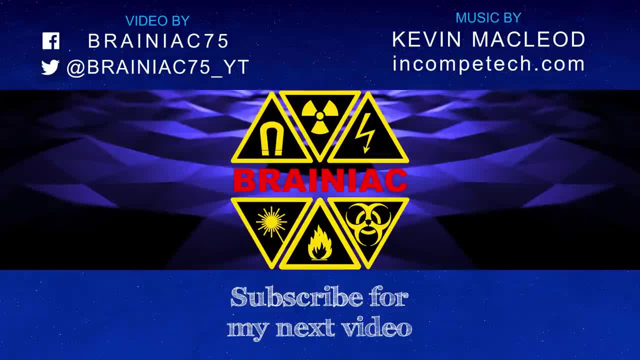 If you did, Then go nuts on that, Hit the thumbs up button to let me know And make sure you are subscribed for the next video. Thanks for watching. Bye for now.